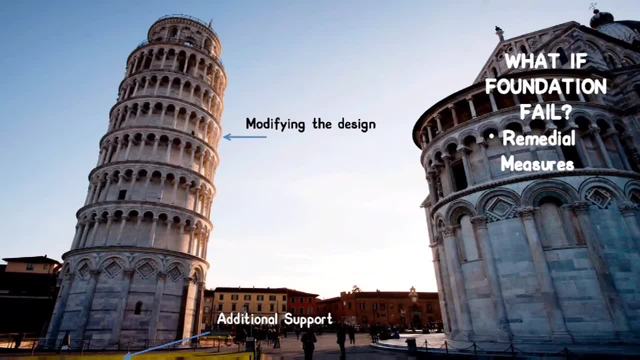 it can carry the load from the superstructure. Now, if the problem is with the soil, then you will try to modify the soil or you will try to stabilize the soil by doing some ground improvement techniques. Now, if all these rectifying measures fail, then we will have no other choice but to abandon the structure. Now, all these. 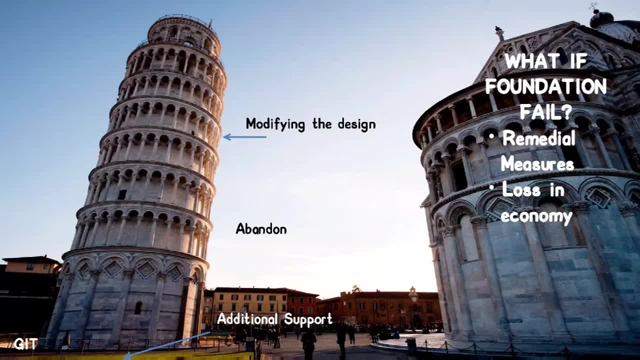 remedial measures will give an enormous loss in economy. So before we start any- that is, before we start constructing any major, massive or cost-consuming work, we'll have to first go to the site and study the site. So we will have to first go to the site and study the site. So we will have to first go to the. 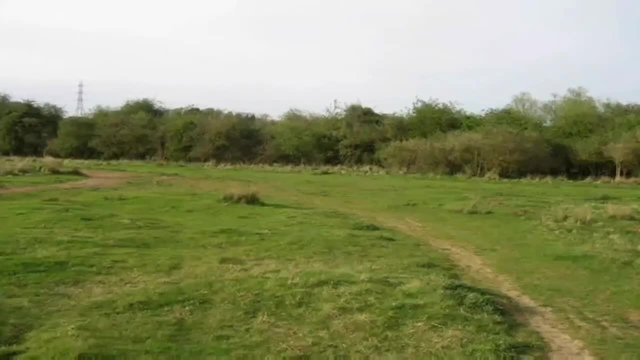 site and study the site. So we will have to first go to the site and study the site. So let's say that we are at a site, That is, we are visiting this site. So the first thing that we will do is that we'll do a. 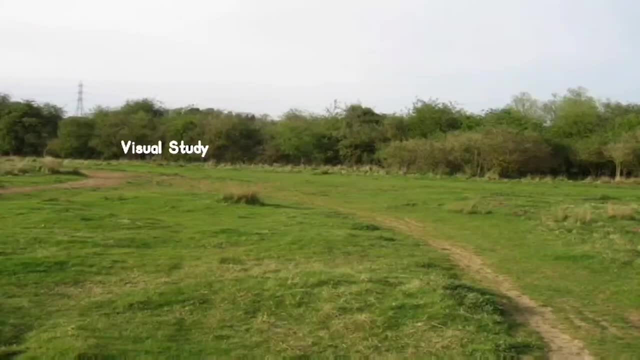 visual study. But with just the visual study, that is, by just observing this site, we will not know what is the type of the underlying soil, What is the strength of the soil, where the groundwater table is located, etc. So for that we will have to do some extensive study. So the all the overall procedure. 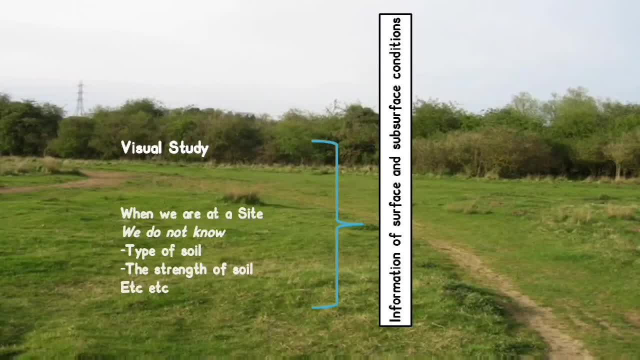 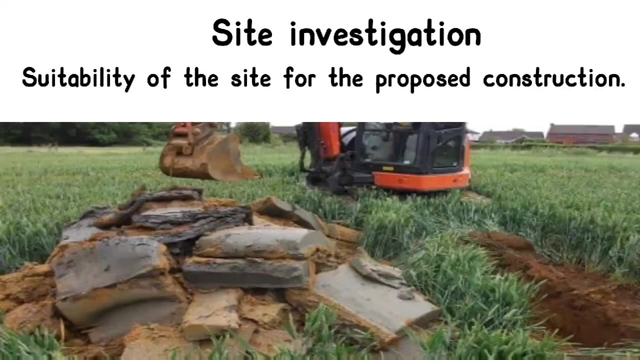 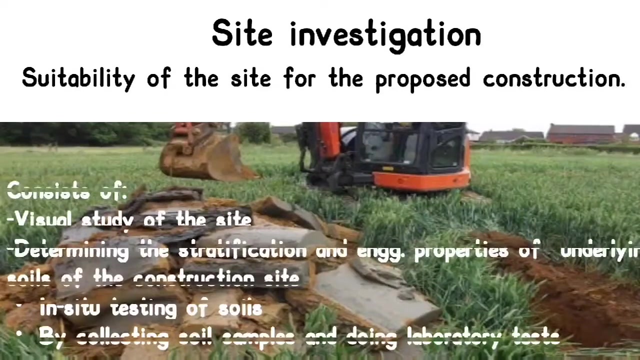 of collecting the information or determining the information of surface and subsurface conditions will be called the site investigation or the soil exploration program. So a site investigation is basically to understand whether the site is suitable for the proposed construction work. The site investigation mainly consists of going to the site. 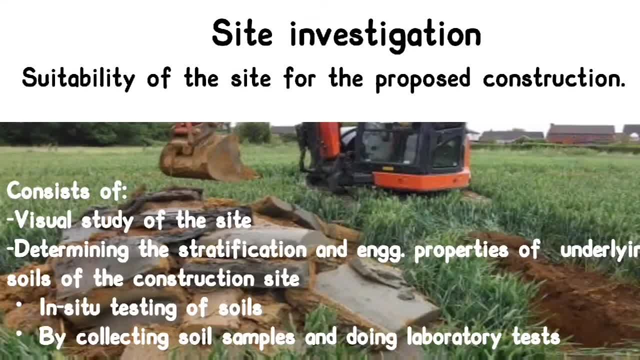 and doing a visual study of it and determining the stratification and engineering properties of the underlying soils. These engineering properties are determined by doing a field test, that is, in-situ test, or by collecting soil samples and by doing laboratory tests. The next video will be on the objectives of soil exploration program. Till then stay blessed, Thank you.